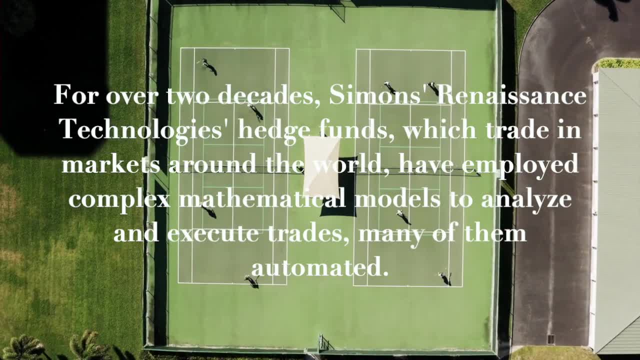 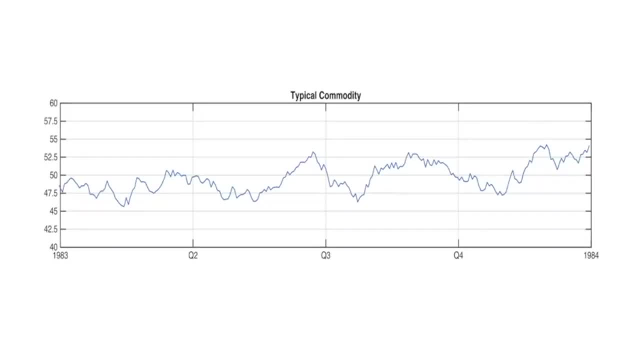 of thing we did back at IDA. You design an algorithm, You test it out on a computer. Does it work, Doesn't it work, And so on. Turns out in the old days- and this is kind of a graph from the old days- commodities. 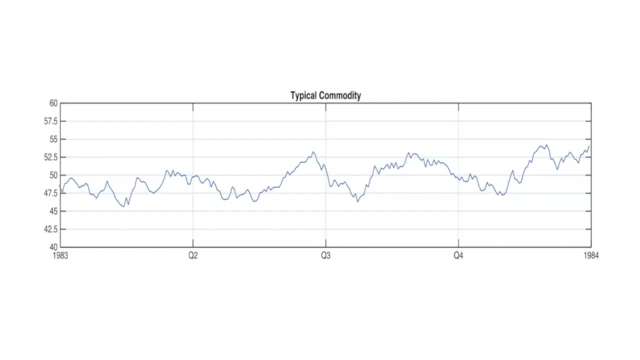 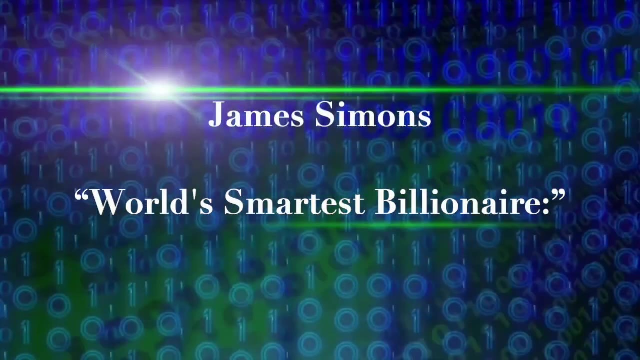 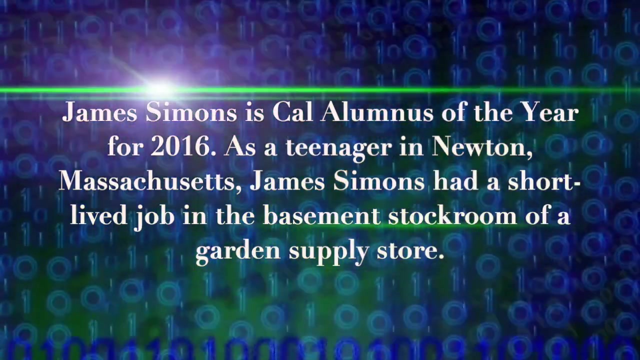 or currencies had a tendency to trend, Not necessarily the very light trend you see here, but trending. It was trending in periods And if you decided, OK, I'm going to predict today by the average move in the past 20 days- there's 20 days. maybe that would be a good prediction and 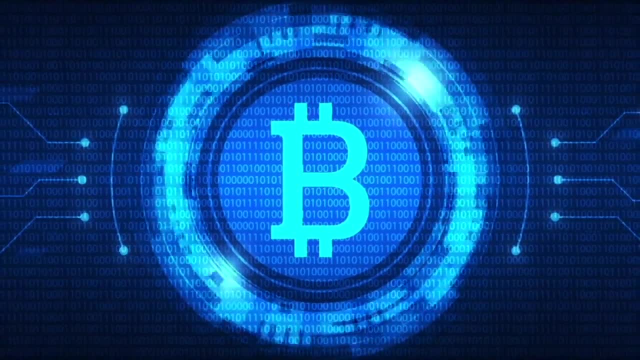 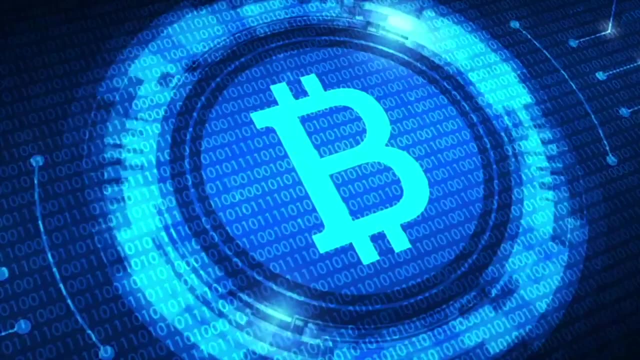 I'd make some money And in fact, years ago such a system would work- Not beautifully, but it would work. So you'd make money, You'd lose money, You'd make money, But this is a year's worth of days And you'd make a little money during that period. 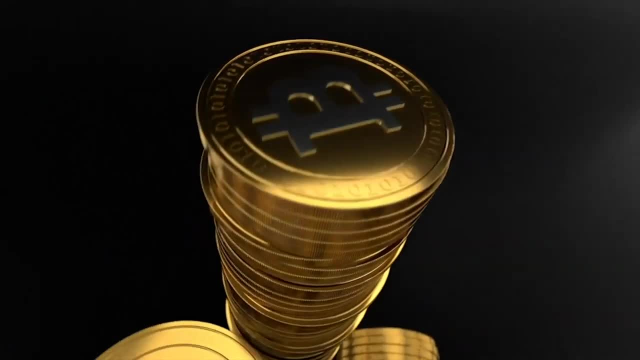 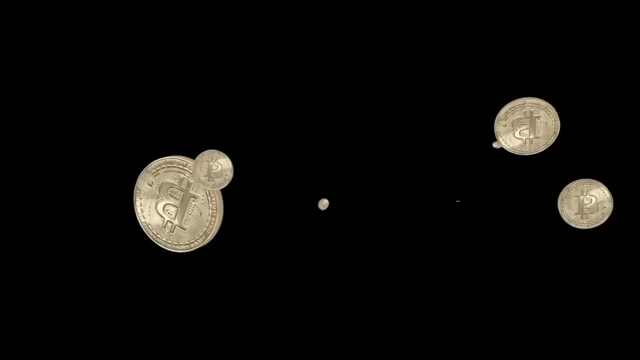 Try all those things and see what worked best. But the trend following would have been great in the 60s and it was sort of OK in the 70s. By the 80s it wasn't such a problem. We stayed ahead of the pack by finding other approaches. 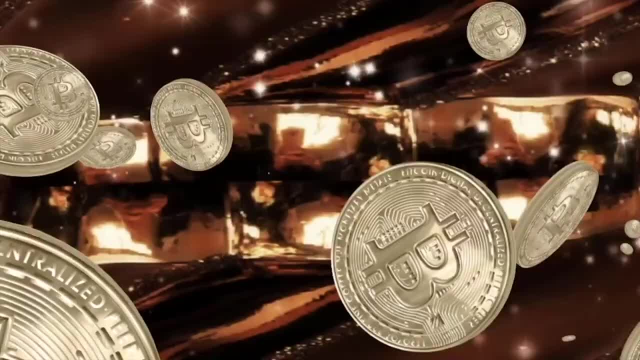 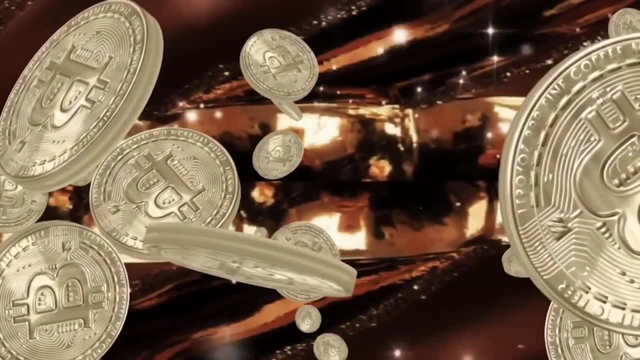 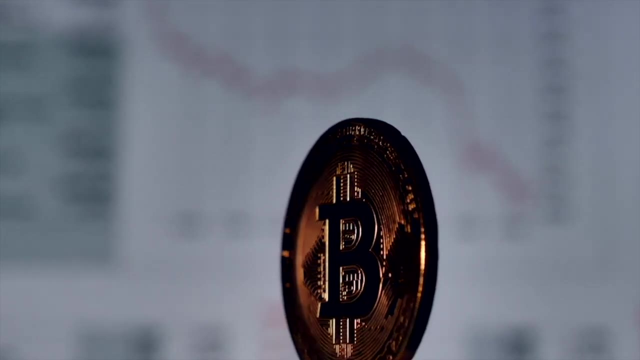 and shorter-term approaches to some extent, But the real thing was to gather a tremendous amount of data And we had to get it by hand. in the early days We went down to the Federal Reserve and copied it- Interest rate histories and stuff like that- because it didn't exist on computers We got. 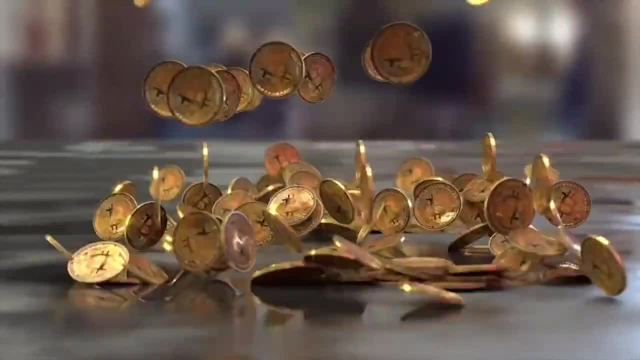 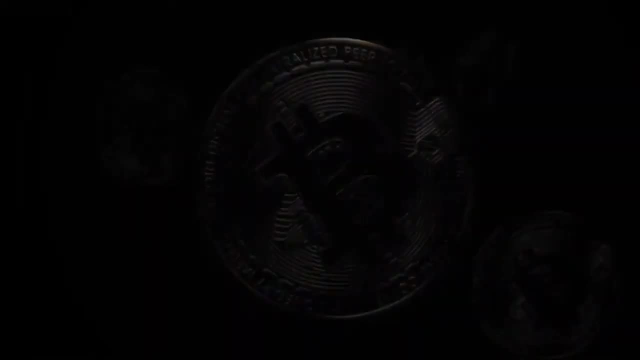 a lot of data and very smart people, And that was the key. I didn't really know how to hire people to do fundamental trading. I had hired a few. Some made money, Some didn't make money. I couldn't make a business out of that, But I did know how to hire scientists because 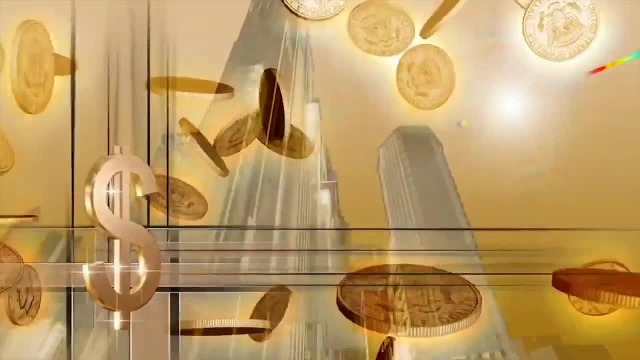 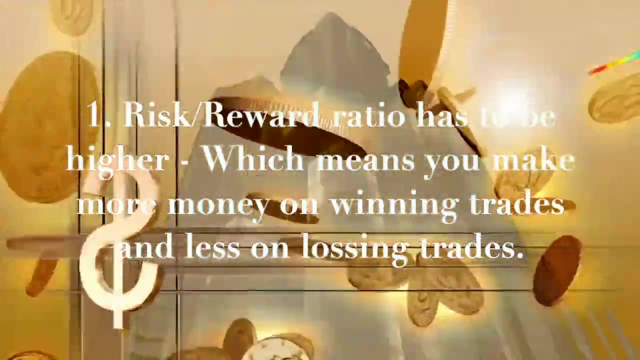 I had some taste in that department And so that's what we did. And gradually these models got better and better and better. Some of it was money. They made a lot of money. I can't say that no one came because of the money. I think a lot of them came because 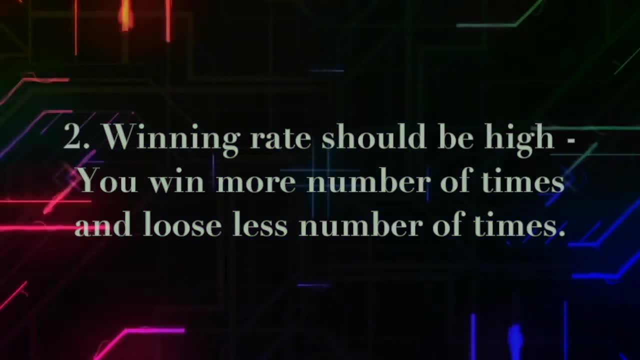 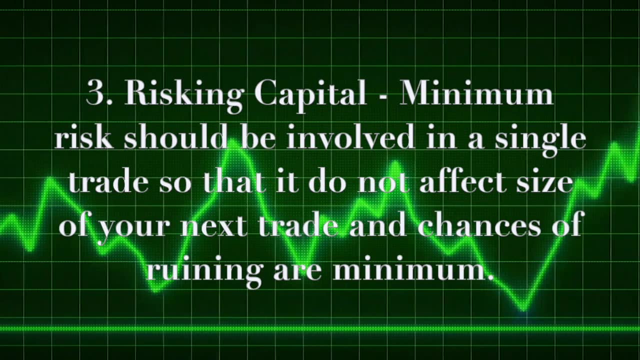 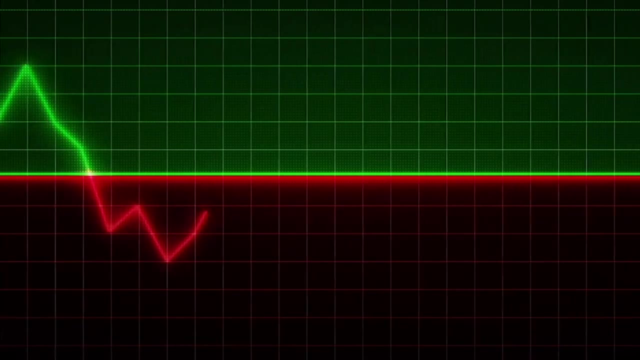 of the money, But they also came because it would be fun. Well, in a certain sense, what we did was machine learning. You look at a lot of data and you try to simulate different predictive schemes until you get better and better at it. It doesn't necessarily feed back on itself the way we did things, But it worked. We take 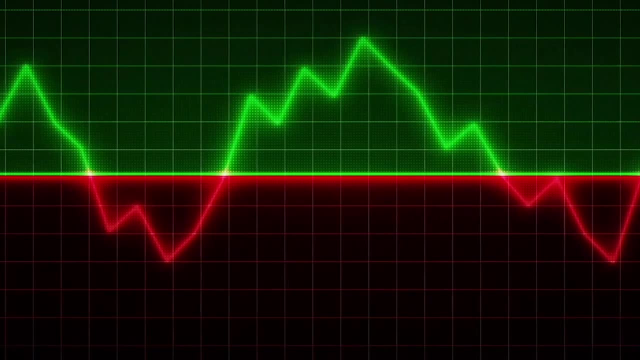 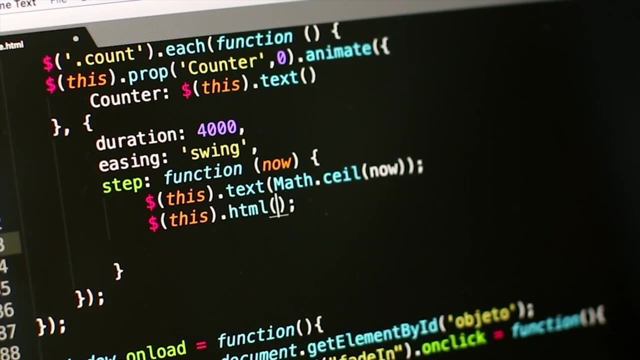 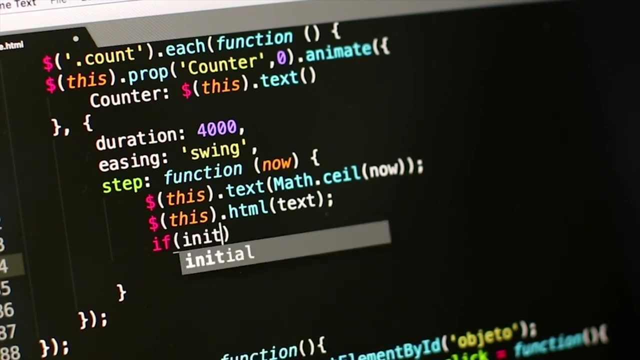 in terabytes of data. We take in a lot of data a day and store it away and massage it and get it ready for analysis, And you're looking for anomalies. You're looking for, like you said, the efficient market hypothesis. Well, any one anomaly might be a random thing. However, if you have enough data, you can. 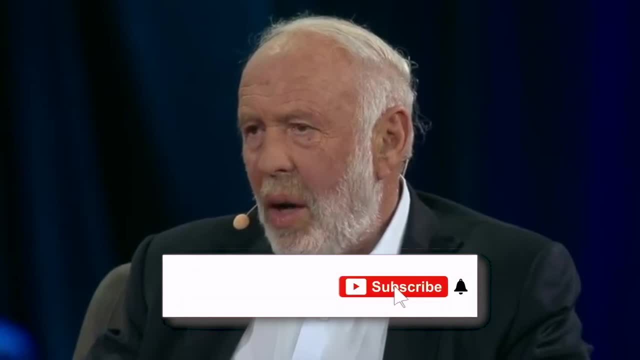 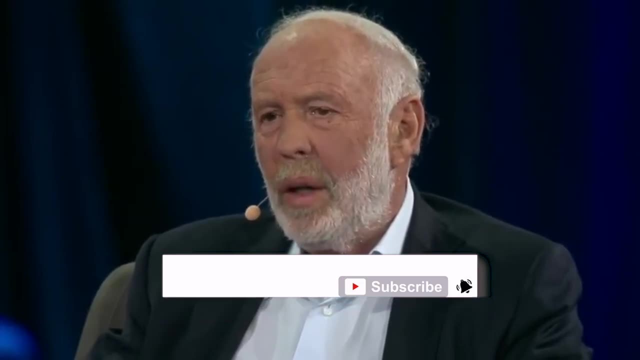 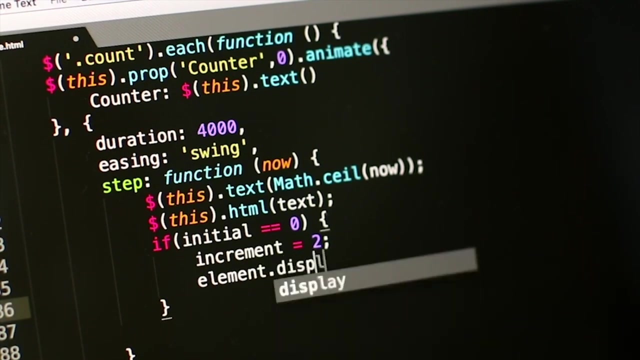 tell that it's not. So you can see an anomaly that's persisted for a sufficiently long time, So the probability of it being random is not high. But these things fade after a while. Anomalies can get washed out, So you have to keep on. 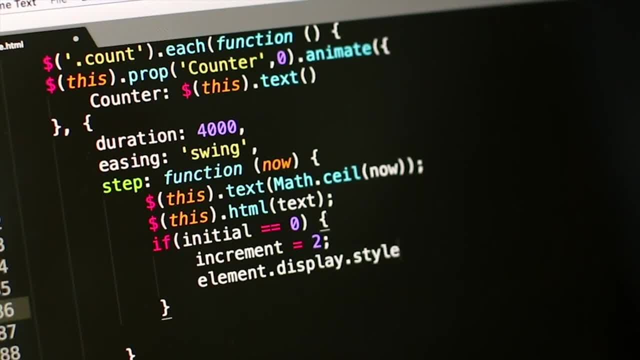 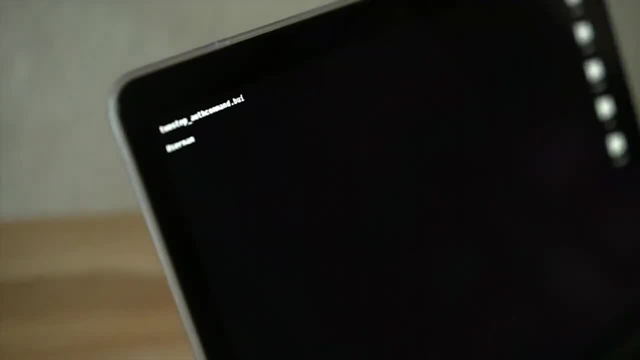 top of the business. Well, actually, I think in the last three or four years hedge funds have not done especially well. We've done dandy, But the hedge fund industry as a whole has not done so wonderfully. The stock market has been on a roll, going up, as everybody knows, And price earnings 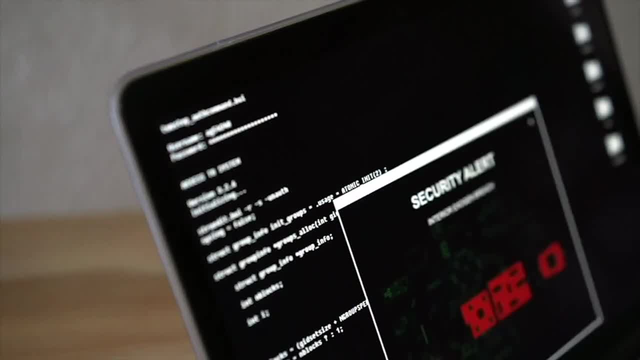 ratios have grown. So an awful lot of the wealth that's been created in the last, let's say, five or six years has not been, It's not been created by hedge funds, So it's just another. People would ask me what's? 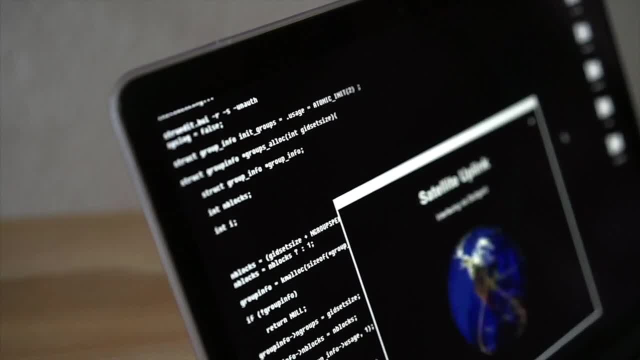 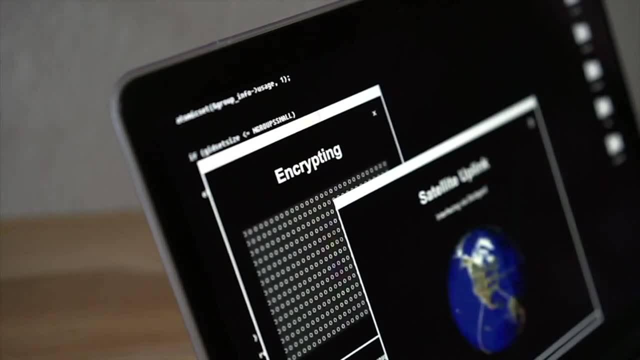 a hedge fund And I say one in 20, which means now it's two in 20.. It's 2% fixed fee and 20% of profits. Hedge funds are all different kind of creatures People got very mad at. 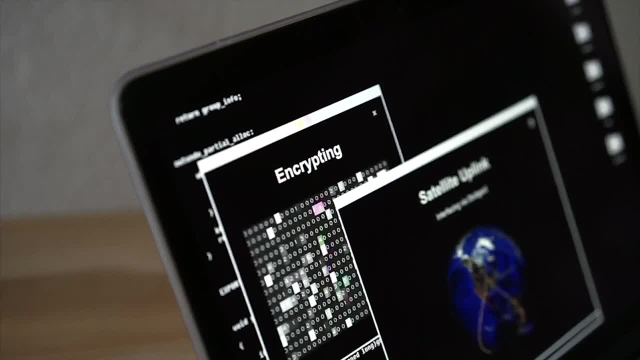 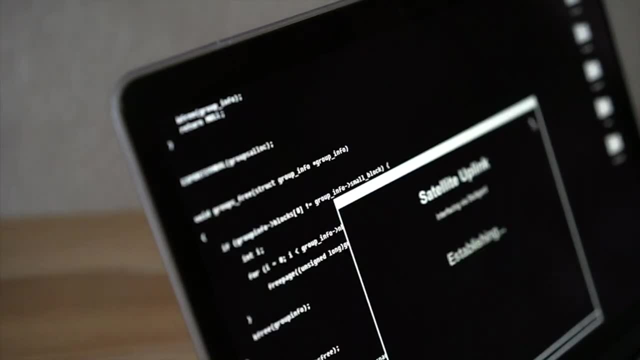 my investors. How can you charge such high fees? I said, OK, you can withdraw, But nope, How can I get more? was what the answer was. How can I get more? But at a certain point, as I think I told you, we bought out all the investors Because 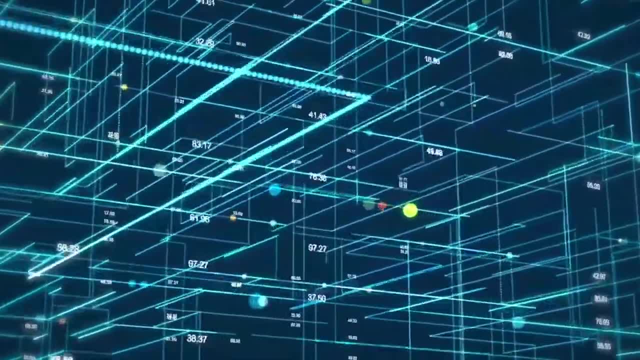 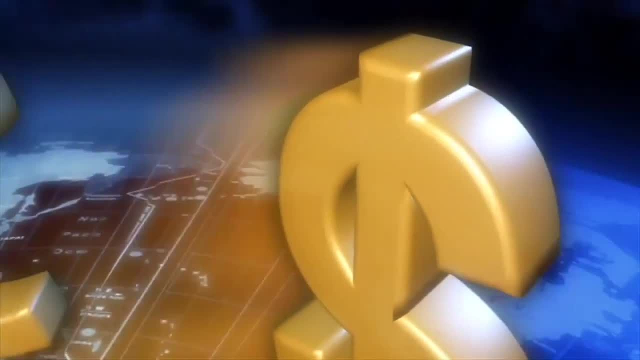 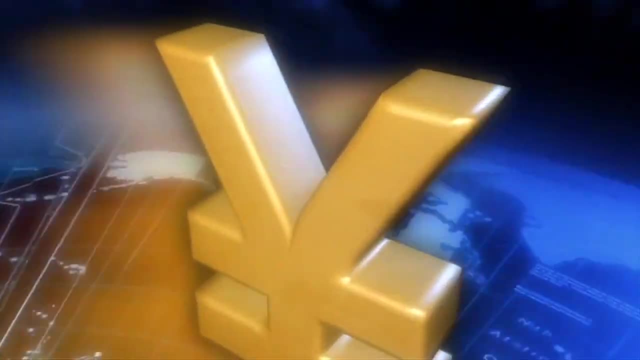 there's a capacity. There's a capacity. It's not just mathematical. We hired astronomers and physicists and things like that. I don't think we should worry about it too much. It's still a pretty small industry And, in fact, bringing in science into the investing world. 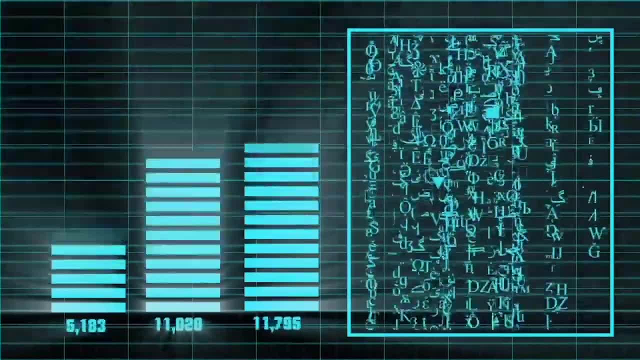 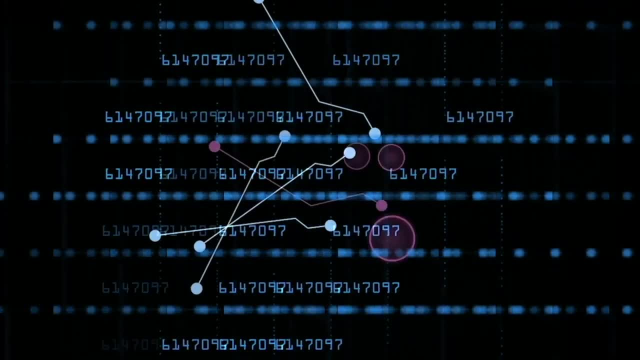 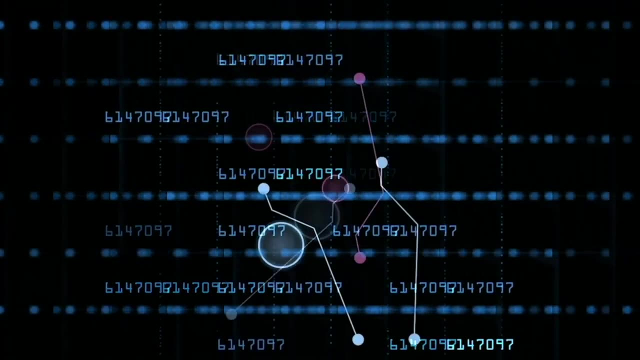 has improved that world. It's reduced volatility. It's increased liquidity. Spreads are narrower because people are trading that kind of stuff. I'm not too worried about Einstein going off and starting a hedge fund. No, Yeah, we are. Marilyn started there. she is up there. A beautiful wife She started. 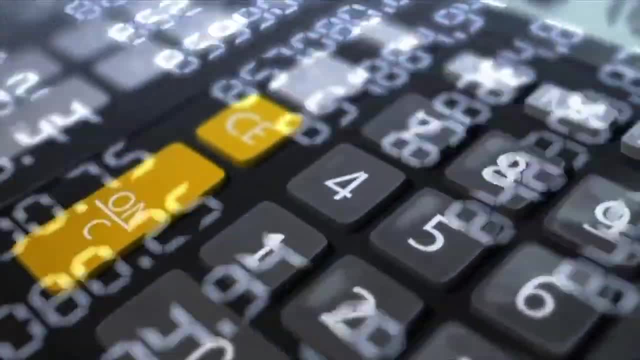 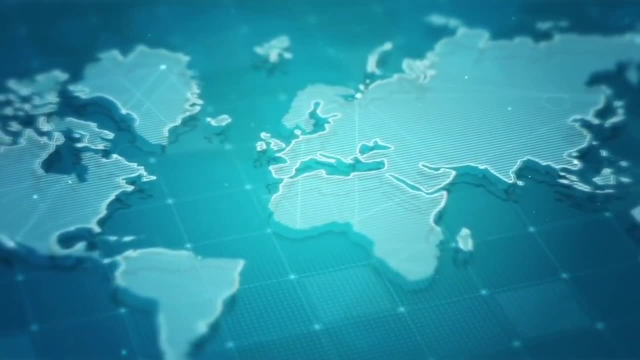 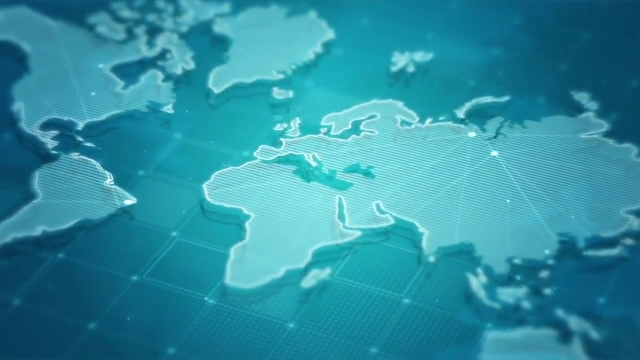 the foundation about 20 years ago, I think 94. I claim it was 93. She says it was 94,, but it was one of those two years. We started the foundation And, just as a convenient way to give charity, she kept the books and 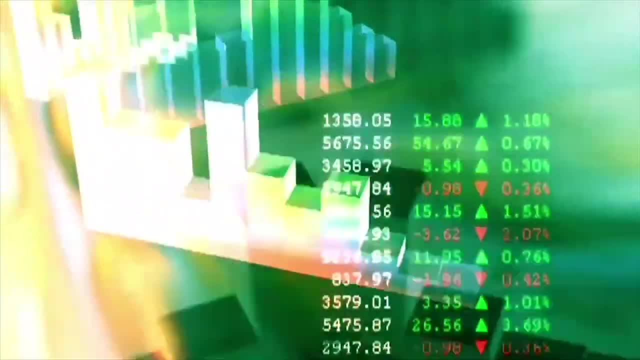 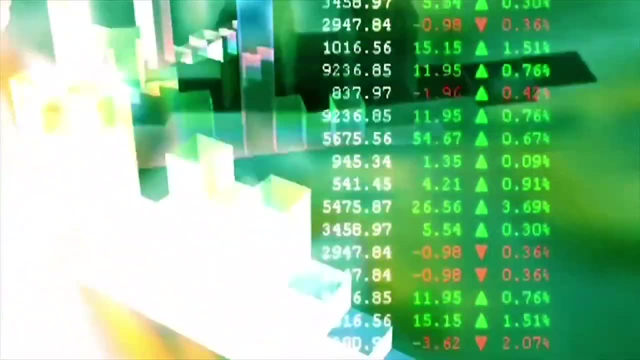 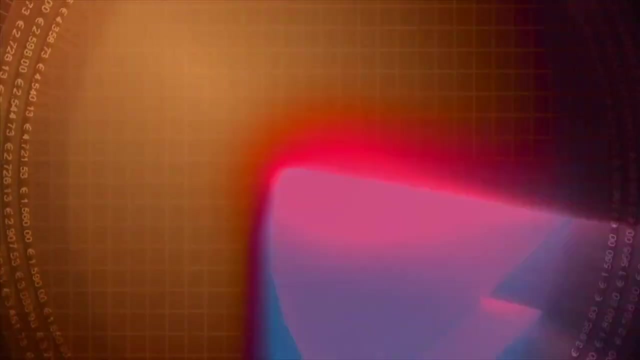 so on, And we did not have a vision at that time, but gradually a vision emerged which was to focus on math and science, to focus on basic research, And that's what we've done, And six years ago or so, I left Renaissance and went to work at the foundation, So that's. 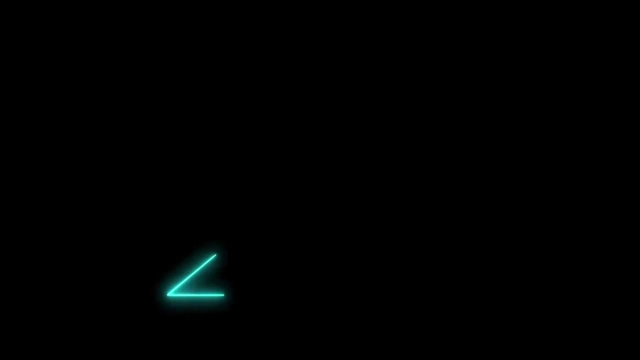 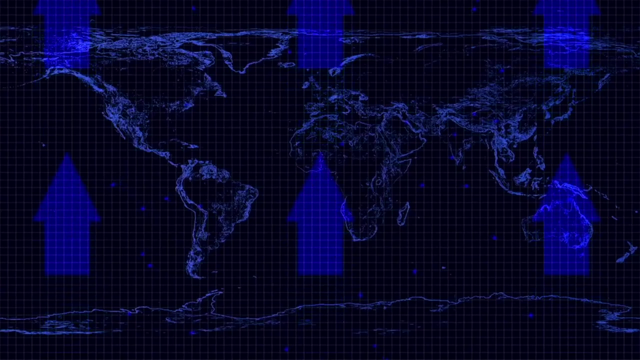 what we do. Instead of beating up the bad teachers, which has created morale problems all through the educational community, in particular math and science, we focus on celebrating the good ones and giving them status. Yeah, we give them extra money, $15,000 a year. 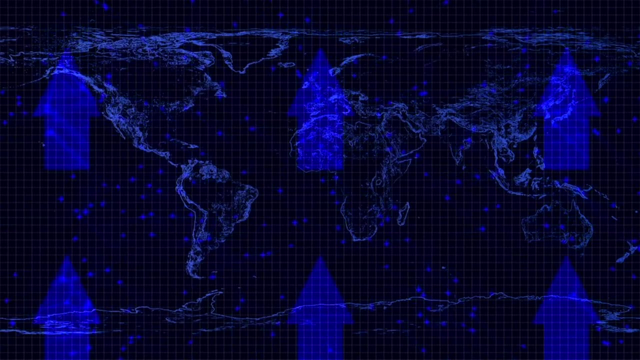 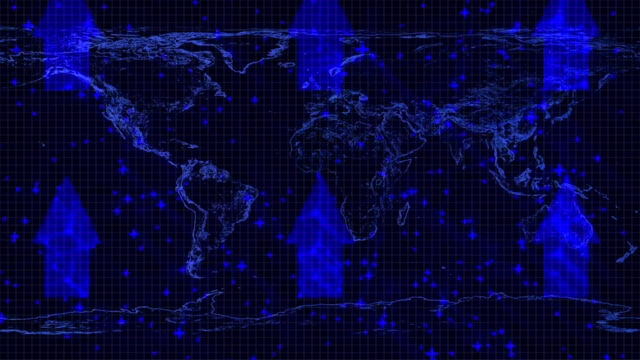 We have 800 math and science teachers in New York City in the public schools today as part of a core. There's a great morale among them. They're staying in the field. Next year it'll be a thousand and that'll be 10% of the math and science teachers. 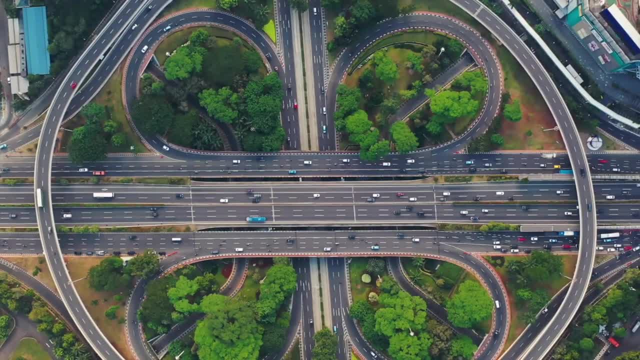 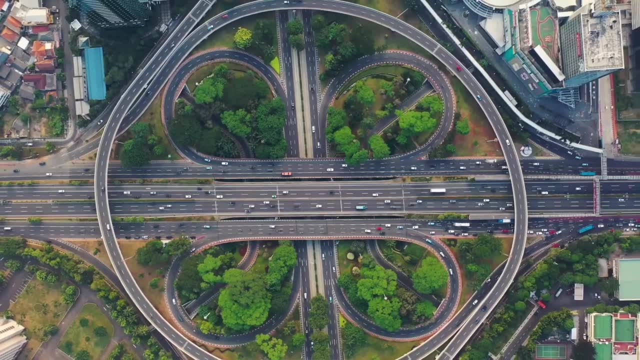 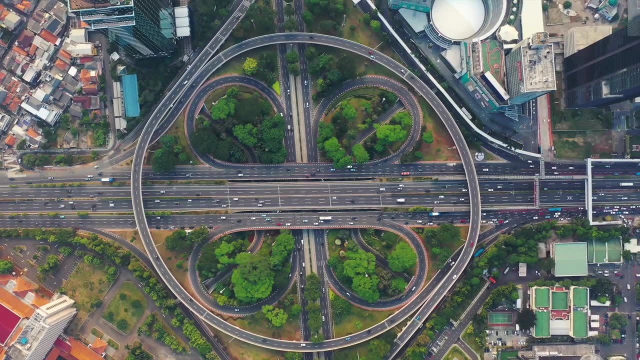 Well, I'll save that for a second and then I'll tell you what you're looking at. So Origins of Life is a fascinating question. How did we get here? Well, there's two questions. One is: what is the route from geology to biology, How did we get here? And the other 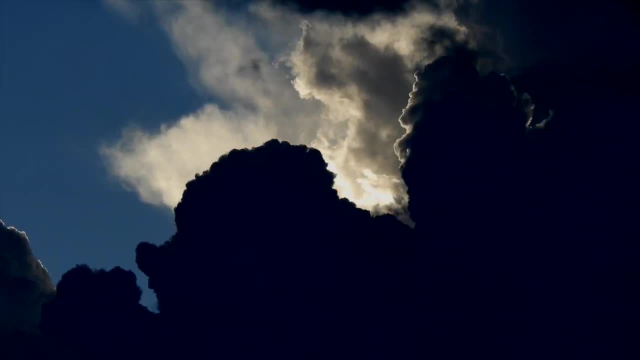 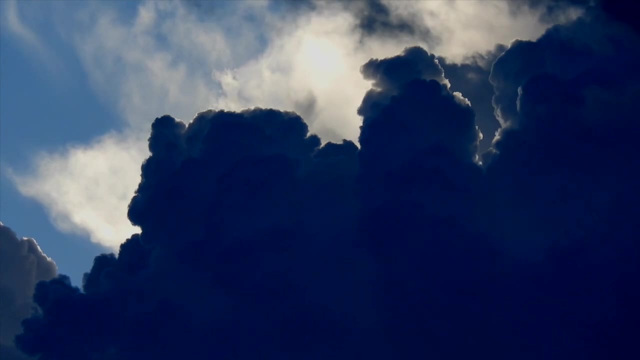 question is: what did we start with? What material, if any, did we have to work with on this route? Those are two very, very interesting questions. The first question is a tortuous path from geology up to RNA or something like that. 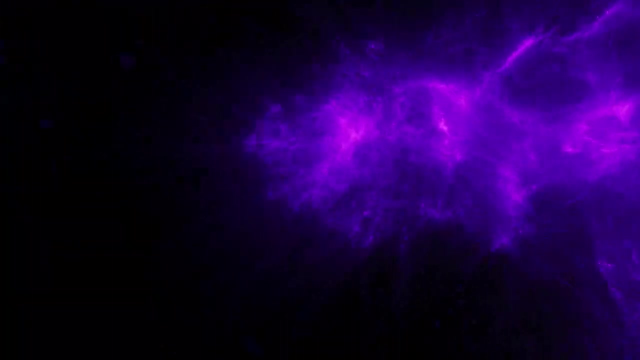 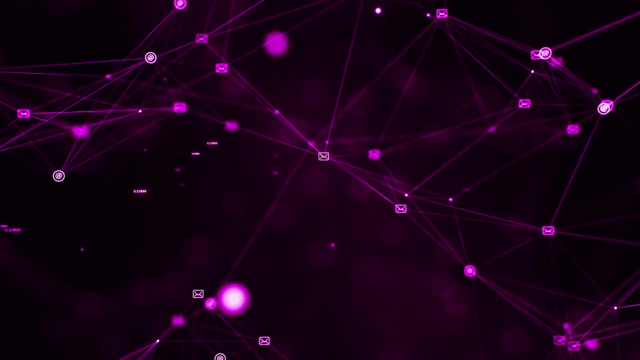 How did that all work? And the other, what do we have to work with? Well, more than we think. So what's pictured? there is a star in formation. Now, every year in our Milky Way, which has a hundred billion stars, about two new stars are created. Don't ask me how. 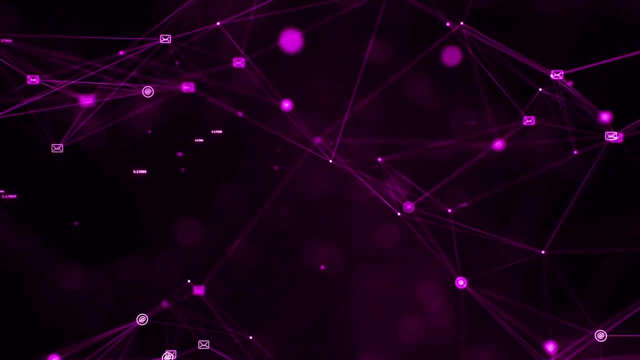 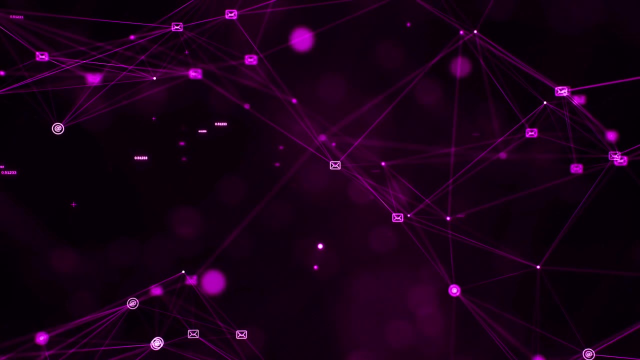 but they're created And it takes them about a million years to settle out. So in steady state there's about two million stars in formation at any time. That one is somewhere along this settling down period And there's all this crap sort of circling around it. 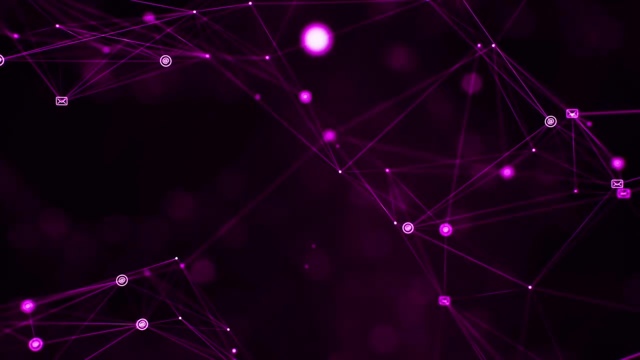 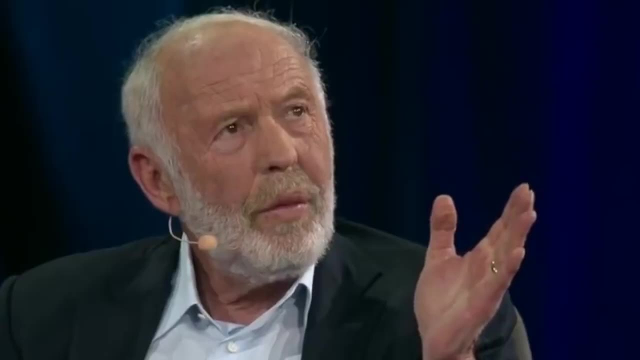 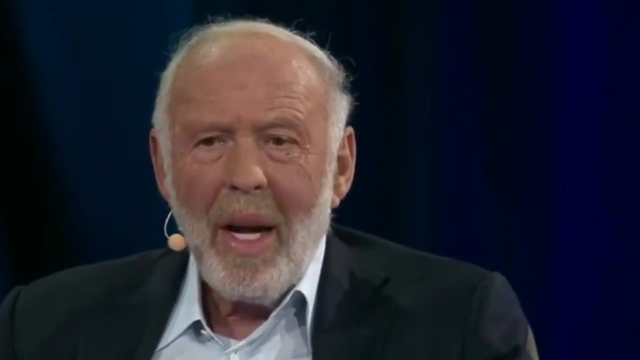 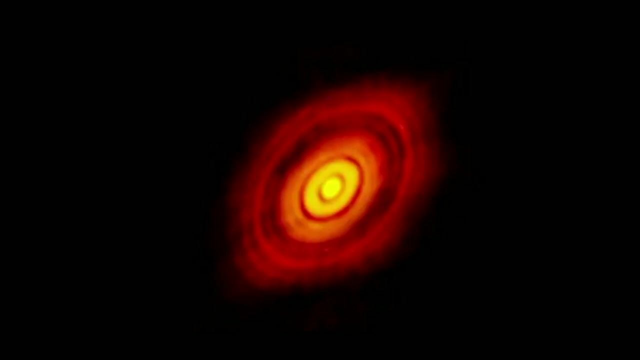 dust and stuff And it'll form probably a solar system or whatever it forms. But here's the thing: In this dust that surrounds a forming star have been found now significant organic molecules, Molecules not just like methane, but formaldehyde and cyanide, things that are the building. 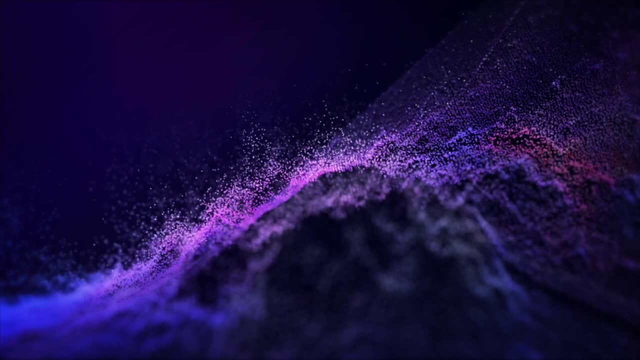 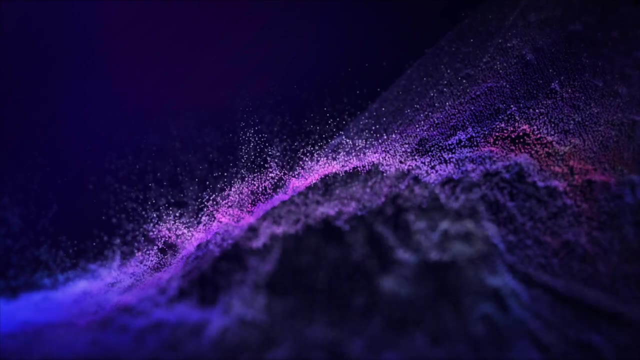 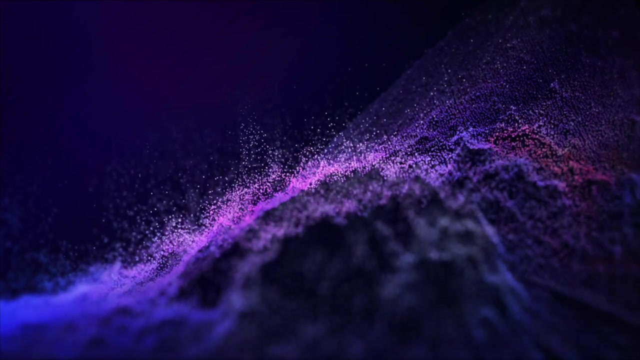 blocks, the seeds, if you will, of life. So that may be typical, And it may be typical that planets around the universe start off with some of these basic building blocks. Now, does that mean, oh, there's going to be life all around, Maybe? 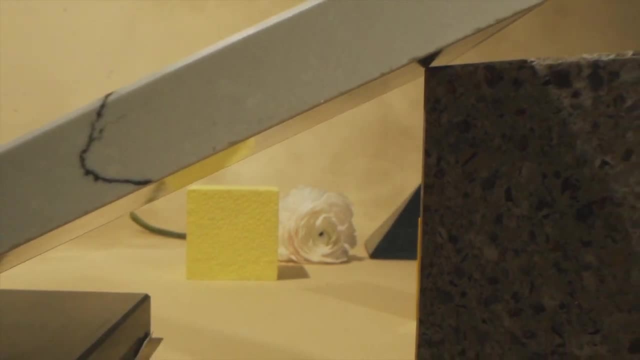 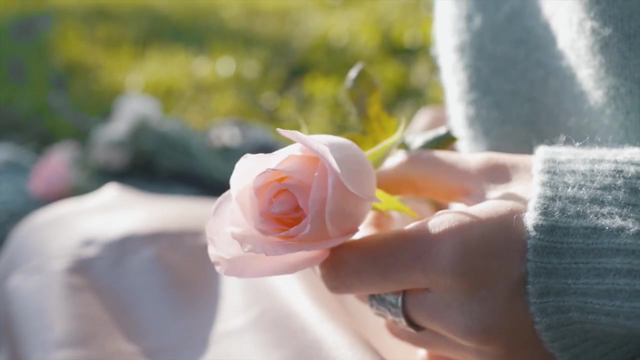 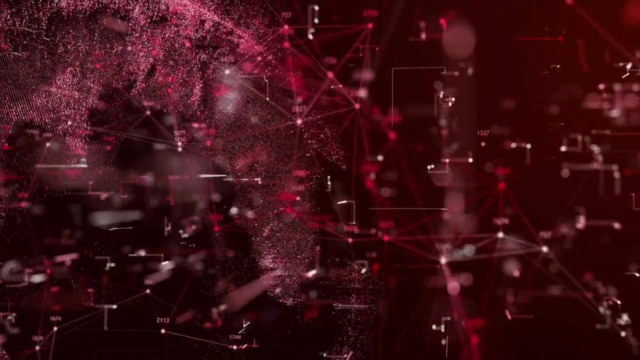 But it's a question of how tortuous this path is, from those frail beginnings, those seeds, all the way to life, And most of those seeds will fall on fallow planets If that path is tortuous enough and so improbable that, no matter what you start with, we could be. 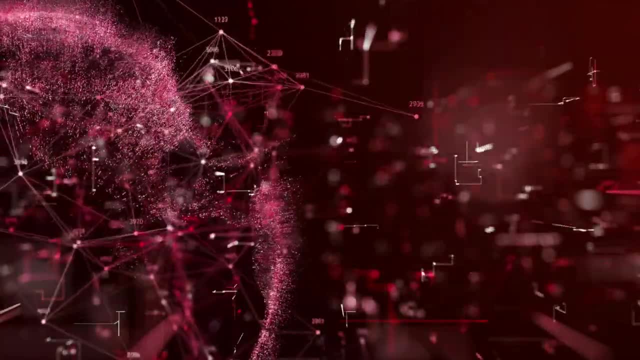 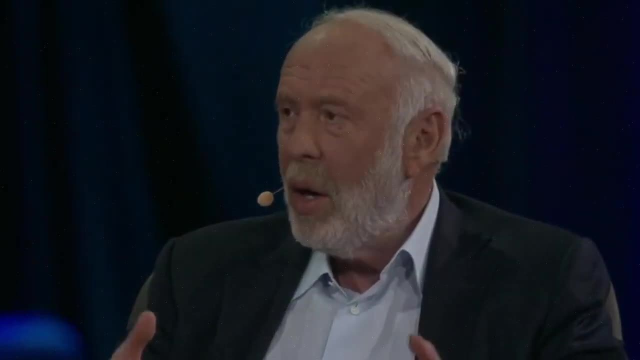 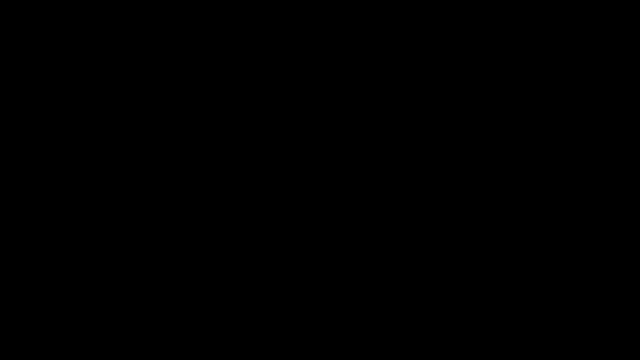 And also we don't know what Shaun is going to think. We don't do that anymore, all kinds of comments that show something as shallow as this on social media and all that kind of stuff. So maybe M&A is taking a piece out of this list where they've completely lost their 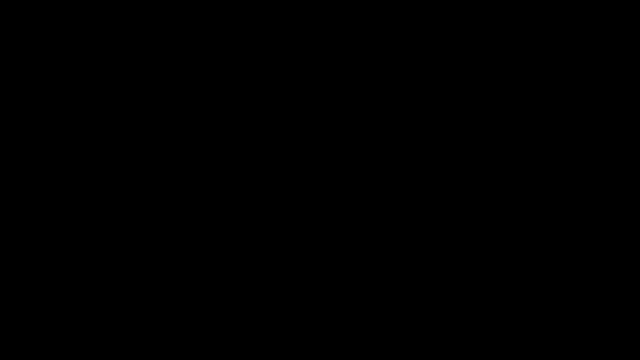 consciousness right at the beginning. Paul Kar�´s Book of History is in our scenario.